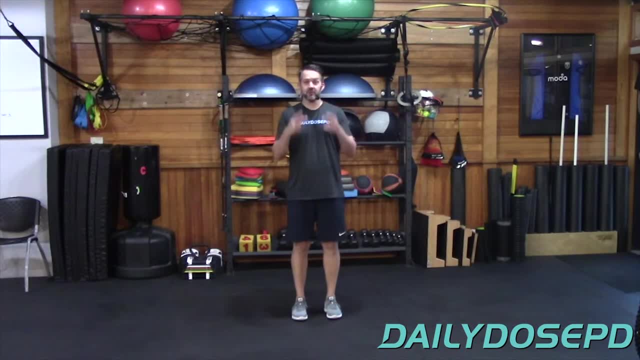 Unbalanced positions. okay, So we're going to do two different phases of this. The first phase is a simple one. I want you to imagine you're looking into a mirror. When I raise an arm or a leg, I want you to do the exact same thing, The exact same thing as you would if you were looking in a 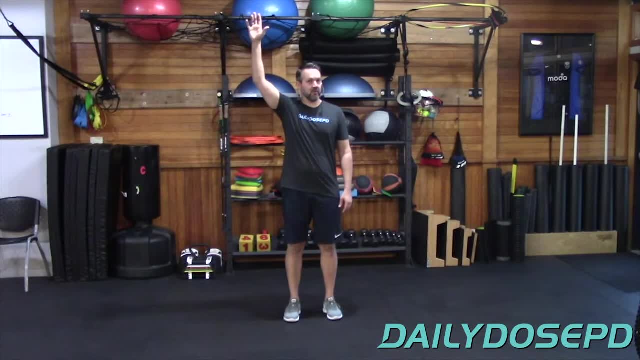 mirror. So if I raise my right hand, your left hand should go up. If I raise my left hand, your right hand should go up, just like you're looking in a mirror. So you're going to move with me. okay, Are we ready? Here we go. 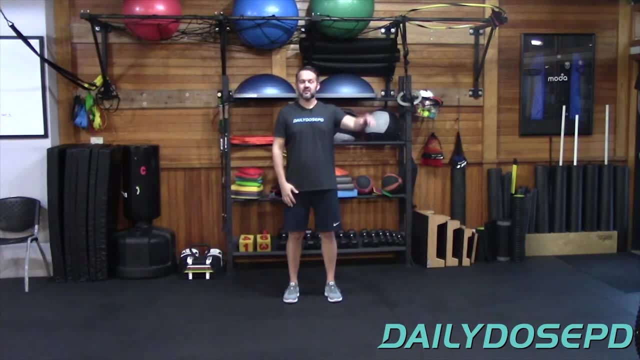 And you're just following what I'm doing and trying to match it step for step and in the same time. So, like I said, if you're in a chair, you can still move. Move your legs close to the same movement patterns as I am. 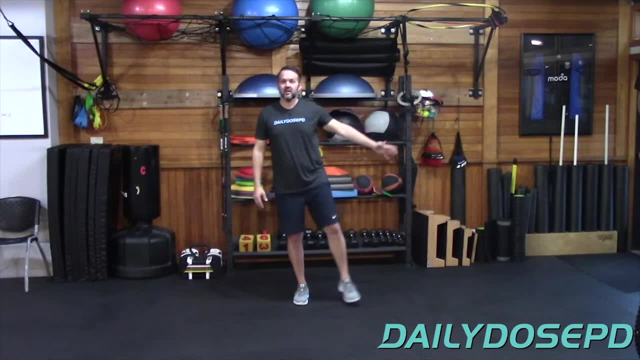 You're still challenging your body. Good work. So that was mirroring. You were having to use your body oriented the same way that I am. Now. we're going to try to flip it, okay, So you're no longer mirroring. Now I want you to raise the exact opposite. 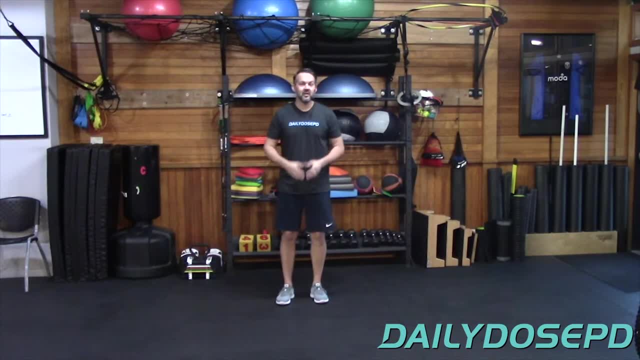 arm and leg that I do. So. if I raise my right hand, you're no longer mirroring me with your left hand. You're actually going to raise your right hand on the other side of your body, up in the air. okay, Same way: if I raise my right leg, you're going to raise your right leg, So it'll. 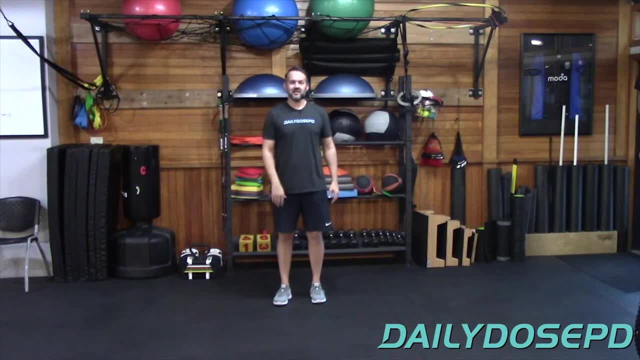 look like it's on the opposite side of what mine is. okay, Are we ready to go? Let's go. So both my left hand and leg are up. Your left hand and leg should be up as well. Both my right hand and leg are up. Your right hand and leg should be up as well.